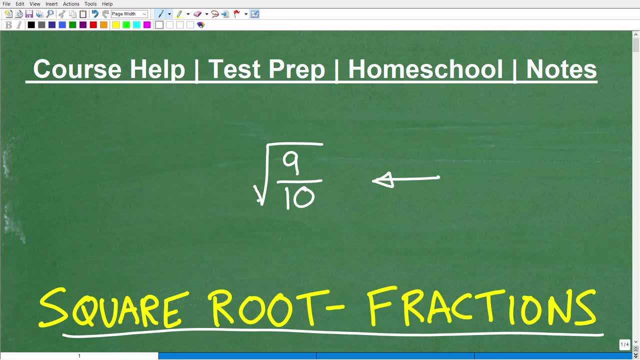 So those of you out there that think you know the answer to this: okay, if this was a pop quiz, for example, and let's say you can get this, if you got this problem right, you would get an A plus in your algebra course and be told you could take the rest of the year off. Okay, imagine, if that was the case. I mean, I mean a lot of you out there be like I would love that. just one question. If I could pass this one question, I won't have to take any more math. So go ahead and see how well you can do with this. Put your answer in the comment section. 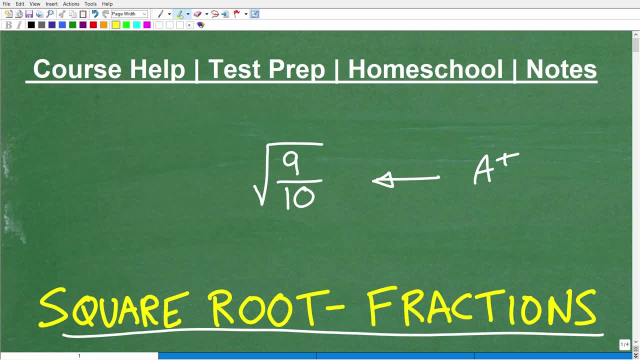 I'll be happy to answer any questions. I'm not looking for a decimal. I'm not asking you to go into your calculator and say nine divided by 10, get some decimal and taking a square root of that, I want you to do this problem without the aid of a calculator and type in your answer into the comment section the best you can. I know you can't put a square root symbol into the comment section, but you know, type it out the best you can do it or just keep it on a piece of paper off to the side and see how well you can do with this particular problem. But I'm going to 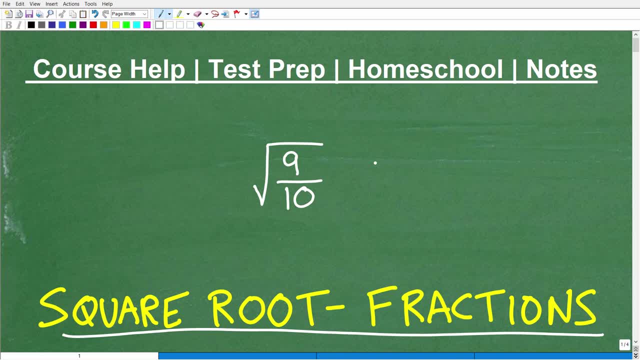 go through this problem and another problem so we can get a quick little mini course on taking a square root of fractions. I'm going to go over all of this thoroughly in just one second, But first let me quickly introduce myself. My name is John. I'm the founder of tablet class math. I'm also a middle and high school math teacher. I'm going to leave a link to my math help program in the description of this video. But if you are having a tough time in math, okay, maybe you don't think you're one of these people that you know has like the natural ability to learn math. 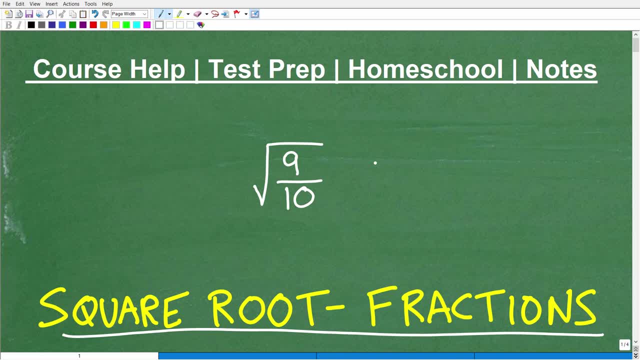 Well, or you struggle with math, or maybe you just hate math, or maybe you don't feel like you're getting enough math instruction, or maybe you're not connecting with your teacher, teachers teaching style. Whatever the case is, I'm going to tell you right now: whatever problem you're having with math, you can be successful math Okay. if there's a will, there's a way. I've been teaching math for decades And I really take the approach to breaking things down and bite size, clear and understandable pieces So anyone could be successful math Okay. so if you're having a tough time or if you just want to get ahead, I can help you out. 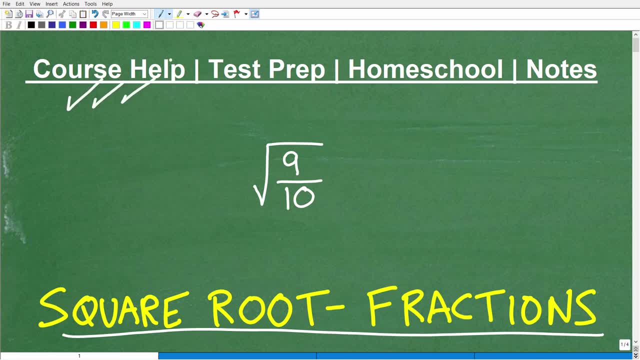 Especially if you're at the middle school, high school or college level in terms of mathematics. Now, if you're preparing for any test that has a math section on it- and there's a lot of them out there. So I'm talking about things like the GED, SAT, ACT, GRE, GMAT, ASVAB, ACCUPLACER, CLEP exam, Alex exam, teacher certification exam, nursing school entrance exam. I can go on and on and on. There's a lot of exams out there have math section on the math. dedicated math sections are on those exams. I can help you prepare for that. 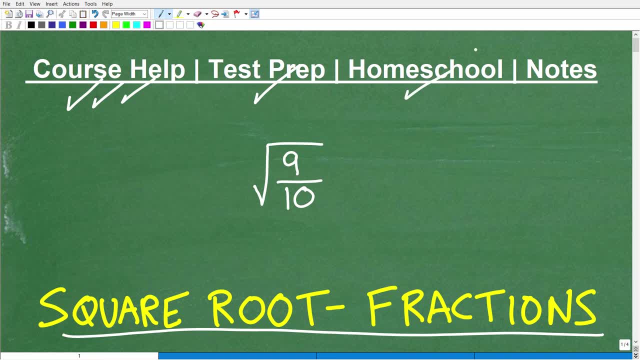 And pass those exams. If you homeschool, you absolutely must check out my full comprehensive homeschool math program and curriculum And if you need some math notes, I'm going to leave links to my math notes in the description of this video. But if you want great grades in math, you must take great math notes. Okay, so start taking better math notes And you'll see your grades just start to skyrocket. All right, let's get to this problem here. So if you had a chance to work on it, you know again, put your answer into the comment section, But 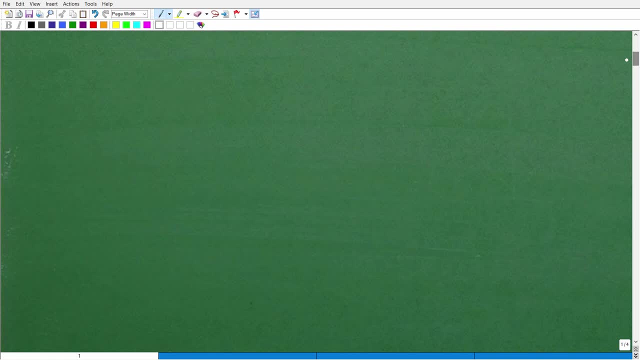 let's get right to it, Okay. so again, if I'm saying take, if I want to know the square root of nine over 10, for example in most algebra classes, what we're being asked to do here is not take nine divided by 10 in your calculator and then take the square root of that and get some sort of decimal. right now, of course, there is a decimal value associated with that, So it's not like it's mathematically wrong, But that's not the whole point. 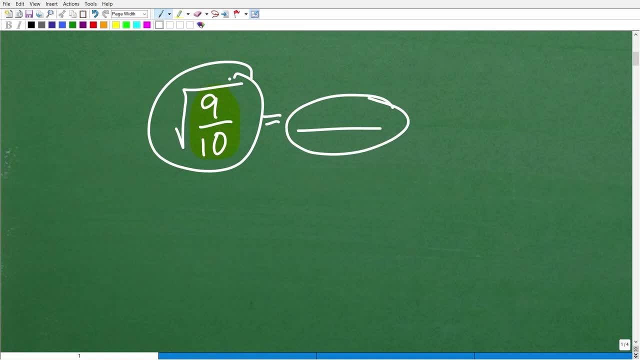 The whole idea here, when we're talking about working with square roots, when we're working with square roots, we need to know this concept right here. So the square root of the fraction a over b is equal to the square root of a over the square root of b. Okay, so this is the property that you need to know. Okay, so we need to keep this in mind And we need to keep something else in mind as well, And I want to show you this by looking at this problem right here. 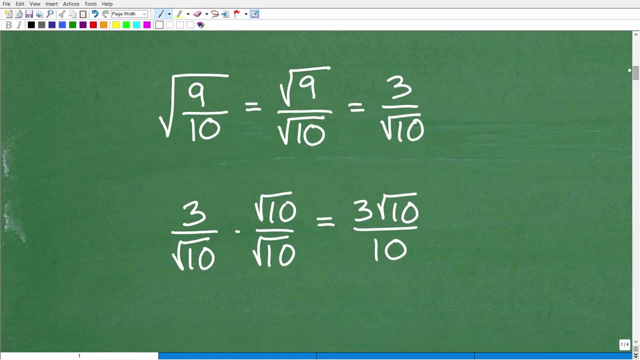 Okay, All right. so let's take a look at this problem. Let's just walk you through it. So I I have the square root of nine over 10.. Okay, nine tenths. So the first thing I'm going to ask myself is: well, okay, nine divided by 10, I can't really simplify this, You know, I can't take nine and divided by 10.. So let's just break this up: the square root of nine over the square root of 10. And the square root of nine, the principal square root, in other words, just the positive square root, is going to be three, And then I have the square root of 10 down here. 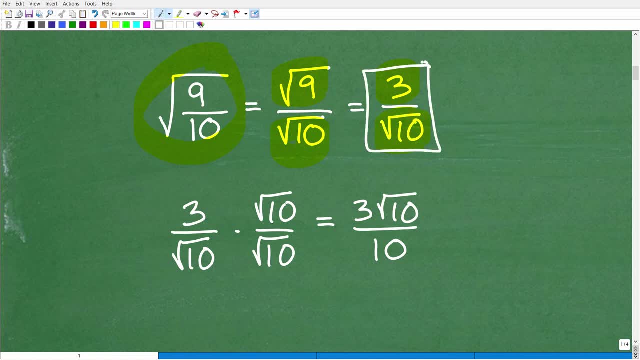 In my denominator. So how many people think that this is the correct answer right here? Okay. so, if you knew that, this is pretty good, Okay. However, I must give you a sad face if you think this is the final answer. Okay, this is not the final answer. This is a good start. However, we have a problem here. Now, what's the problem? Well, we have a square root in the denominator. we're not allowed to leave our answers with the square root in the denominator, what we call an irrational number. 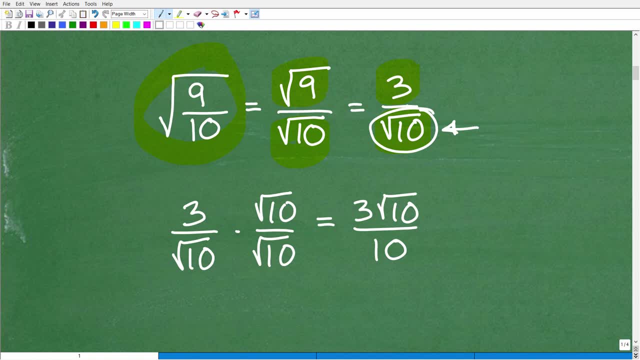 So we have to do something called rationalize, we have to fix this up. So three over square root of 10.. That's what we want. Okay, that's what we. how we broke up this fraction. That's good, But we just need to rewrite this in a better way. So the way we can get rid of this square root, the square root of 10 in the denominator is: I can multiply the denominator by the square root of 10.. But if I multiply the denominator by the square root of 10, I also have to multiply the numerator by the square root of 10.. Now just look, look at this. 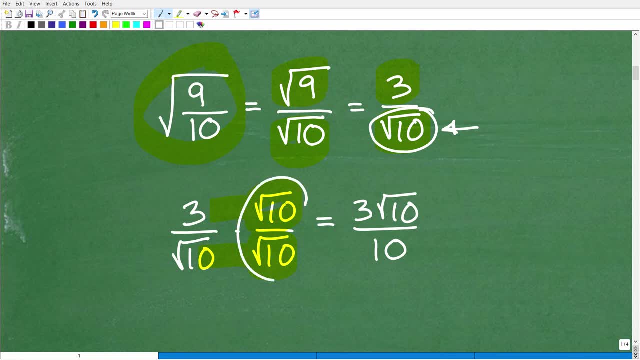 What's going on here? What's the square root of 10 divided by the square root of 10?? Well, this whole thing, anything divided by itself, is simply one. Okay, so this is just a one. So I'm really multiplying this by a fancy one, So I'm not breaking the problem. So somebody out there might be thinking: aren't you changing problem? No, I'm just being creative here And I'm multiplying by a fancy one. But when I do that, though, the advantage is this: the square root of 10 times the square root of 10 is what? Well, it happens to be the square root of 100.. Okay, when you take 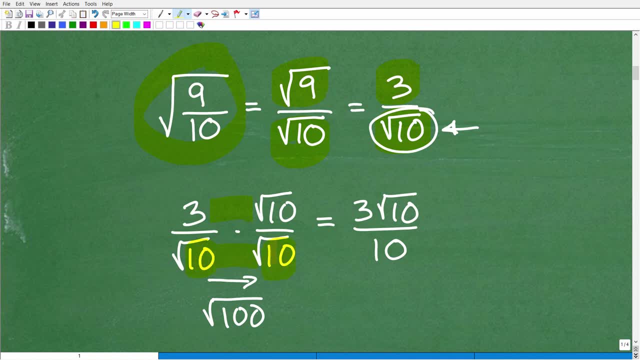 this: when you're multiplying square roots together, we multiply the numbers inside the square root, So that's going to be the square root of 100.. And the principal square root of 100 is 10.. Okay, and so that's what we want. We want to get rid of any square roots in the denominator, But then I have three times the square root of 10.. I could just write it just like this, And this is the final answer: All right, so how many out there got this right? If you did get this right, boy, I tell you I am impressed. I must give you an awesome. 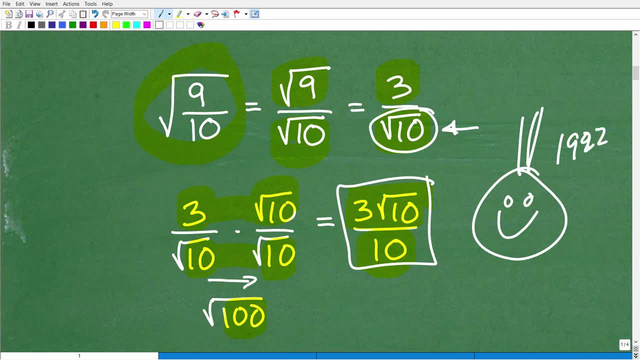 1982. That's not 1922. I don't think they had any Mohawks back in 1922. Maybe they did, I don't know. Look at that. I can't even write 1982.. 1982 Mohawk and an A plus. Matter of fact, I would just say go. 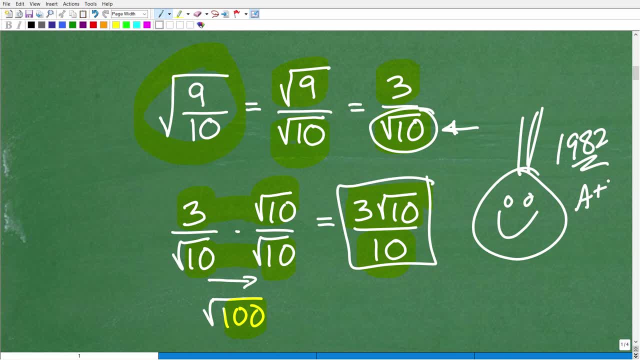 home, And I'll see you next year in your math class. I don't know what you're doing. You must be watching that guy on YouTube. But nice job, Okay, so that's good stuff, That. if you actually knew how to do this, then that's, that's very, very good. But let's go ahead and take a look at another. 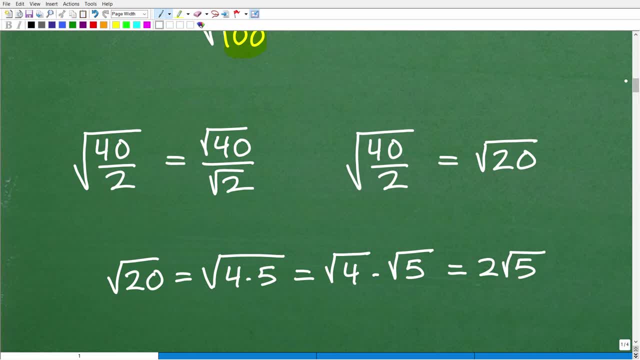 problem here and see how you do with this. Okay, Now you can see I have all the work written out for these two problems, But we're going to take a look at the square root of 40 over two. Okay, so this is a fraction as well, But when I'm looking at this I'm like, okay, you just 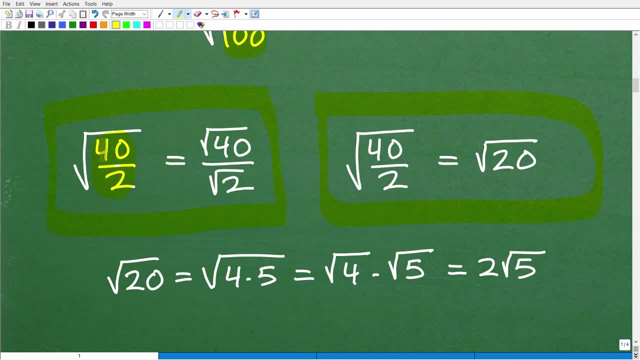 you know, taught me Mr YouTube math man: 40 over two. I can break up the numerator and denominator, So I couldn't write it this way: The square root of 40 over the square root of two. So this is one. 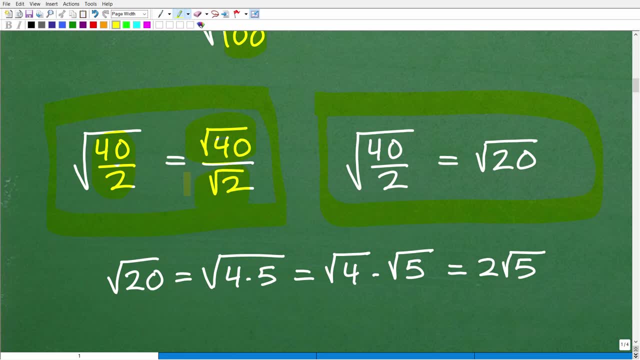 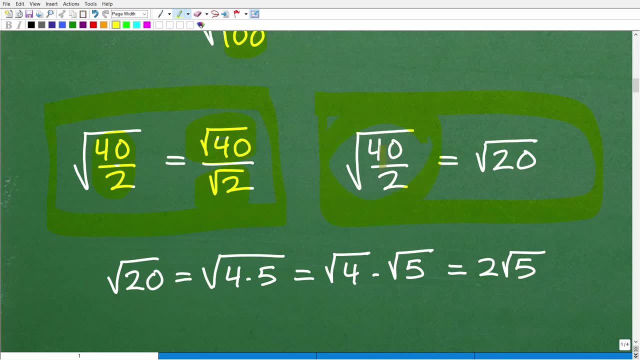 know This is one way we can go, But we can also go this way: square root of 40 over two. Well, 40 divided by two is 20.. Okay, so I'm like, well, maybe I could just simplify this, And 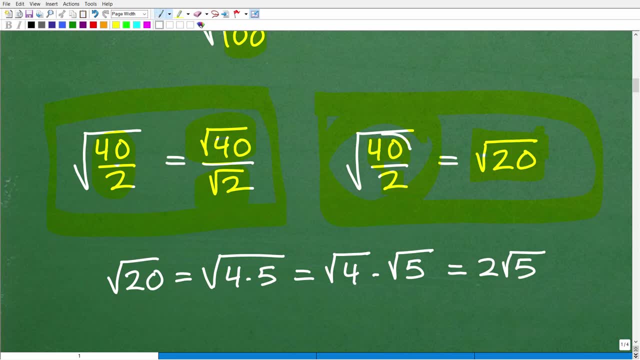 that's exactly what you want to do. So when you can divide these fractions, like in this case, 40 divided by two, that's what you want to do, But here, this is not the final answer. Okay, this square root of 20 is is not fully simplified. 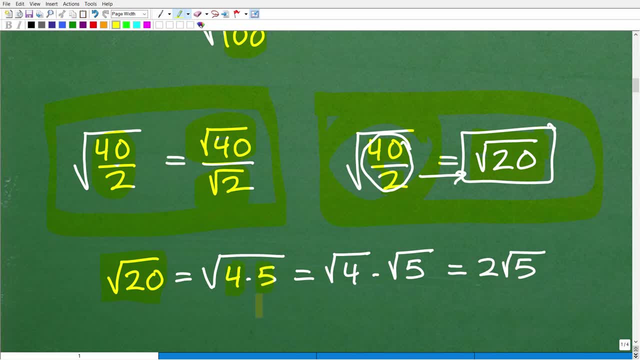 so i can break up 20 as 4 times 5. okay, so this is uh, and what we're talking about here is simplifying square roots. so if you're not really sure what i'm doing, i have additional videos in my pre-algebra and algebra playlist, or maybe you just want to sign up for like my algebra. 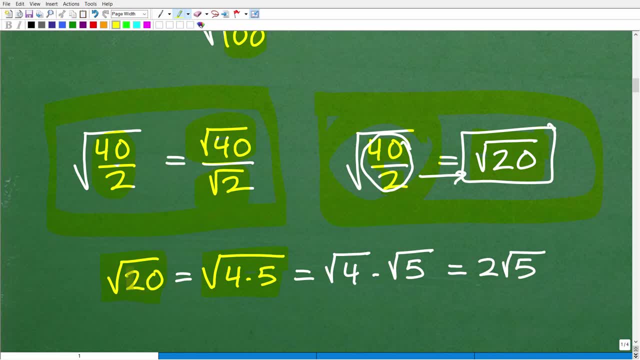 courses to really learn this stuff. but hopefully you can see, the square root of 20 is the same thing as the square root of 5, and now there is a, a, um, another property of square roots. well, this right here, the square root of 4 times 5. i can kind of pull apart this big square root into two. 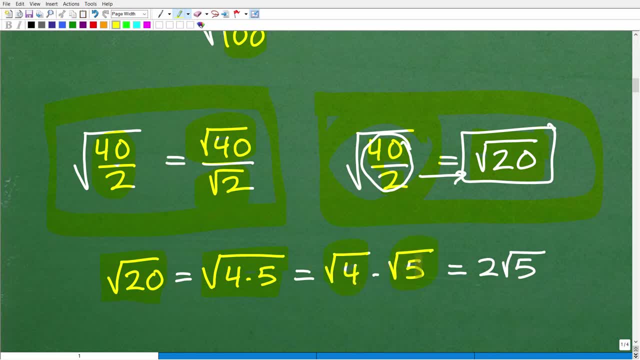 small square roots, so i can write this as square root of 4 times the square root of 5, and, uh, this is advantageous, because now i could take the square root of this 4, which is 2. okay, so that's 2 square root of 5. this is the final answer. so if you're not really you know um 100, follow me on. 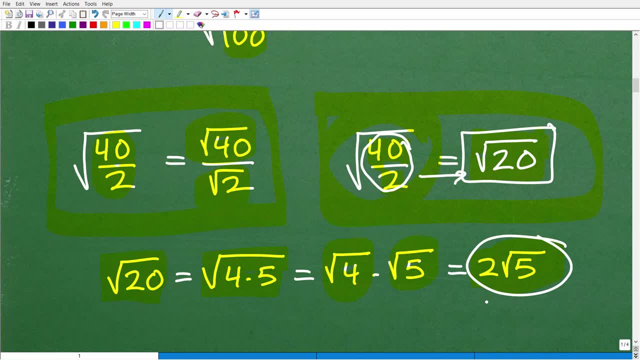 this. then you just got to do some additional review on how to simplify radicals. there's a. you know i'm kind of going a little bit quick and, um, don't want to put too much. in this video we're really kind of focusing on simplifying uh, fractions and you can see that this way. if i went this way, let's take a look at if i went this- 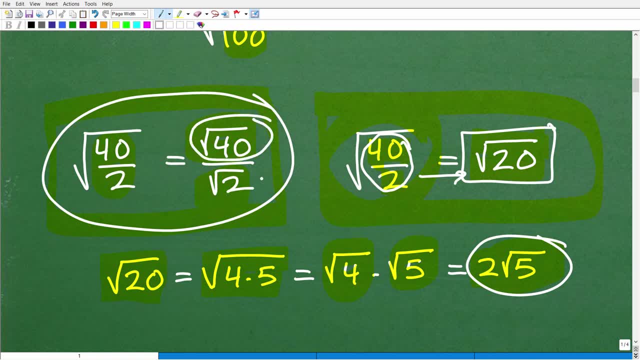 route. okay, well, i would have to simplify the square root of 40 and then i'm going to have to deal with this square root of 2 in the denominator. okay, then i would have to rationalize somewhere along the point. this would be a lot, a lot of work here. okay, you would still get the right answer, but 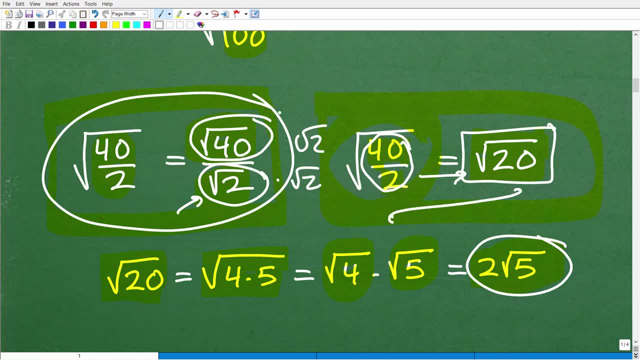 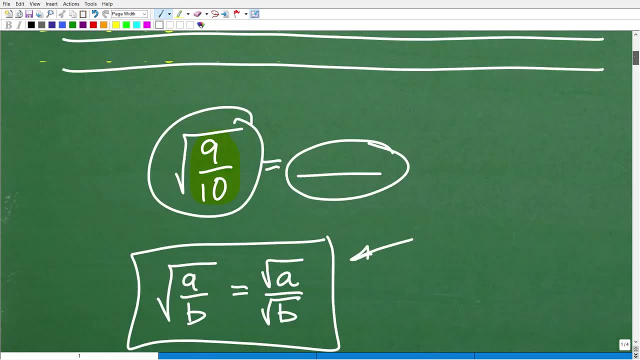 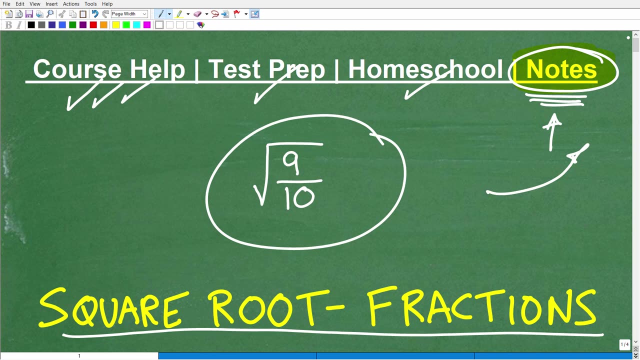 if i went this route. okay, this work is a lot less than doing all this work, okay. so again, when you're faced with taking the square root of a fraction, okay, you want to evaluate what you know, what the deal is, and then take the most effective route. uh, forward. but anyways, uh, hopefully this little video helped. 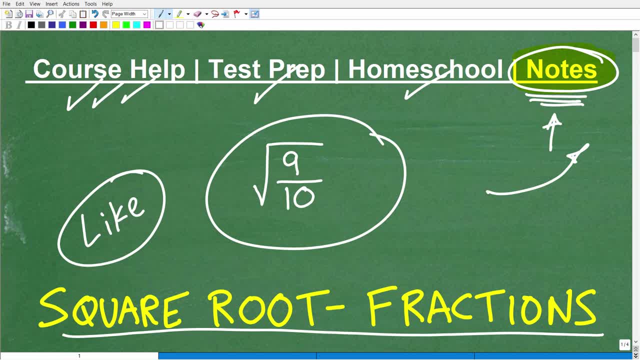 you out and if that is the case, go ahead and smash that like button. that definitely helps me out and if you're new to my youtube channel, hopefully you'll uh consider subscribing. i've been on youtube for 10 plus years, have over a thousand plus math videos, math videos, basic math, to. 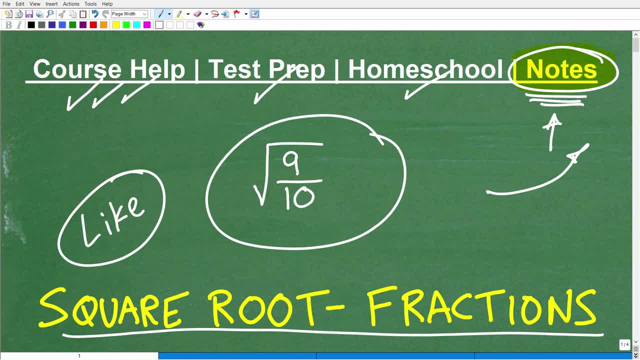 advanced math like calculus and everything in between. i mean, uh, it's taken me that many years to post. uh, well, i think right now i have like 1300 videos. i don't even count. what i do is, i just teach from my- uh, you know my heart every day really trying to help all of you out there be successful in math. there's 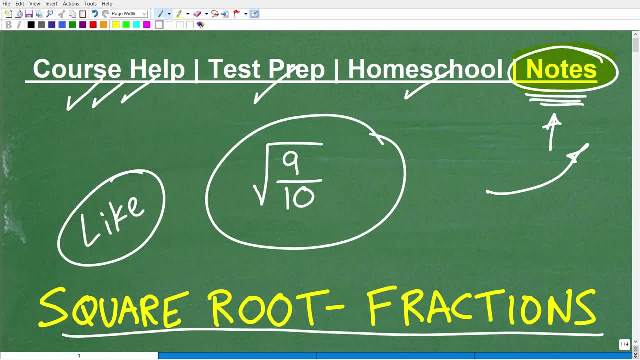 nothing worse. you know, you've been teaching this. i've been, you know, uh, teaching math for such a long time. i hear, you know, all the success stories, but i also hear some very, um, you know to me kind of stories. i hear a lot of adults especially, you know, in their 50s, 60s, even 70s, even in their 80s. 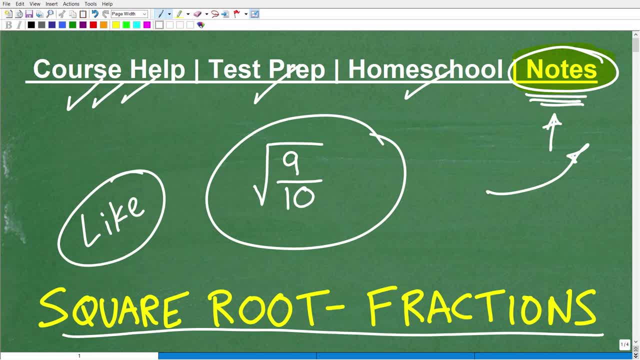 um, and maybe even younger students as well. i mean, i've heard so much and, and what i'm talking about is people saying you know what? i never pursued math because some math teacher back in 1965 told me i was bad at math. or 1978 there was some teacher that says you know what? you're really not. 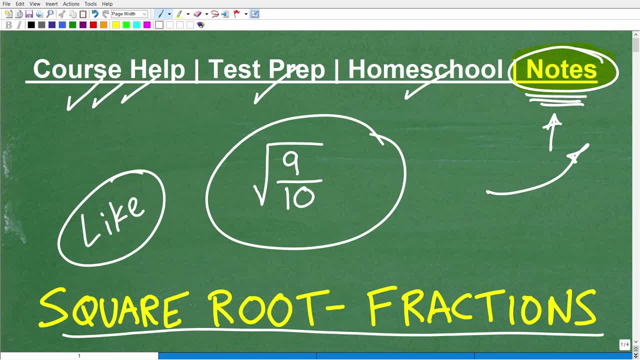 good at math. you should stick with this and that's really. um, you know, any teacher that tells you anything like that is doing a good job of teaching. you know, and i think that's really a disservice to you, okay, and i'm just telling you right now, most of you out there can do so. 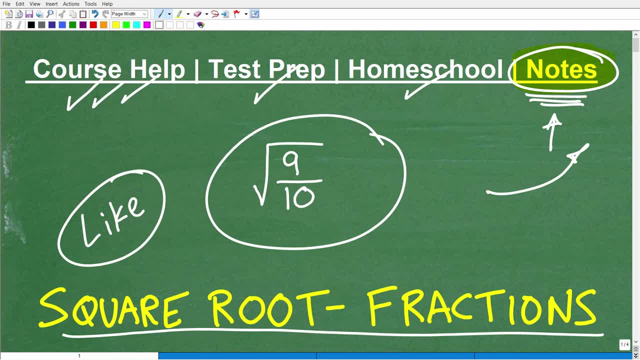 much better in mathematics. you just really got to find the right instruction. so if you've always wanted to learn math and be successful math, i'm telling you right now you can. okay, and unfortunately you know a lot of people have been robbed of their- you know- interest to pursue, maybe, engineering. 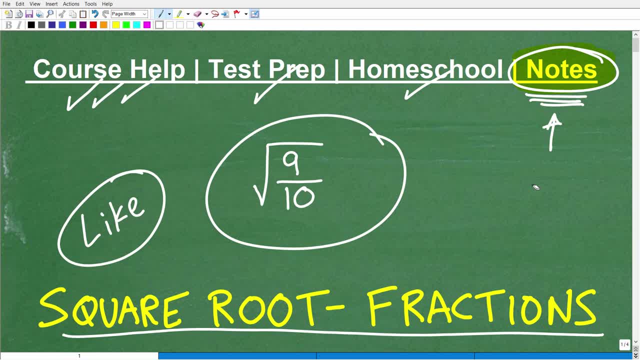 degrees- whatnot? because they don't think they can do the math. okay. so if you're interested in being a scientist, an engineer, but you're scared of the math, listen, stick with it. okay, you can do this stuff. is it easy? no, does it require work? yes, but it's not beyond anything that you can do. so 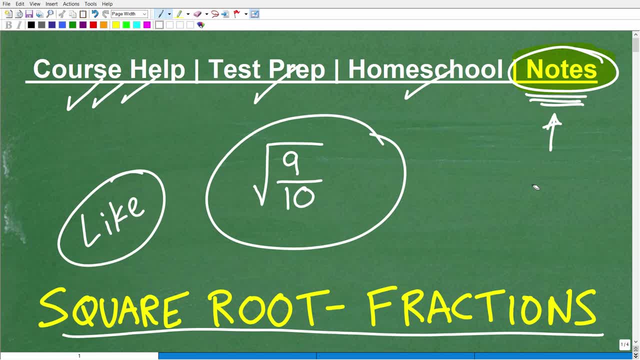 anyways, with that message in mind, if i'm helping you out, please take advantage of all my content, but my best math help will always be within my math help program, okay? so, with that being said, i definitely wish you all the best in your mathematics adventures. thank you for your time. and have a great day.